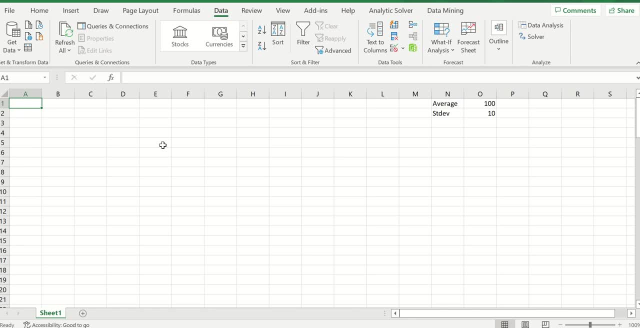 Is everything to walk you through. this is in the book, starting on the bottom of page 565.. But for those of you who are visual learners, let's just do a quick look at this, Go to data And then under data analysis, and if you don't have data analysis, that means you need to add the analysis tool pack option and go look at the bottom of 565.. 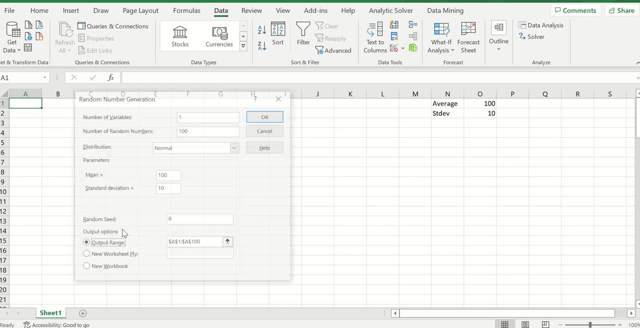 It'll show you how to do that. Come to random number generator. Random number generator for Excel really is saying that you want to produce some information. All right, you want to produce some random numbers. In this case, there's only one variable that we're working with, right. 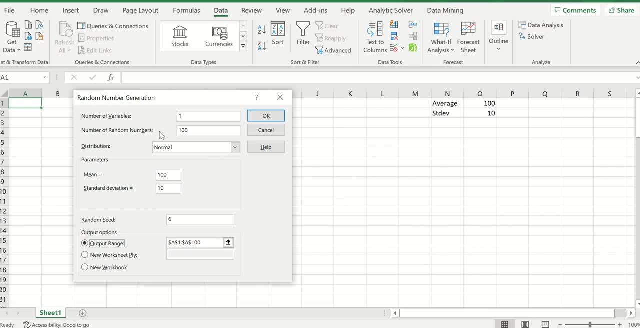 It's just the demand. each month, I want to produce 100 random numbers. You're going to have to type these things in. It probably will not pop up for you. We are thinking that this is a normal number, This is a normal distribution. 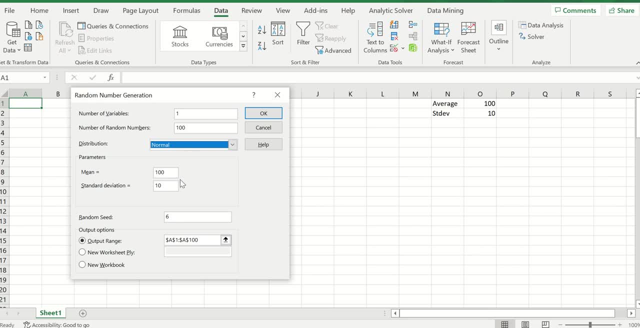 Okay, it's a normal distribution. And when you click on normal distribution, it's going to say: I need Excel, wants a couple of parameters, It wants to know the average and it wants to know the standard deviation. It also wants a seed to get started. 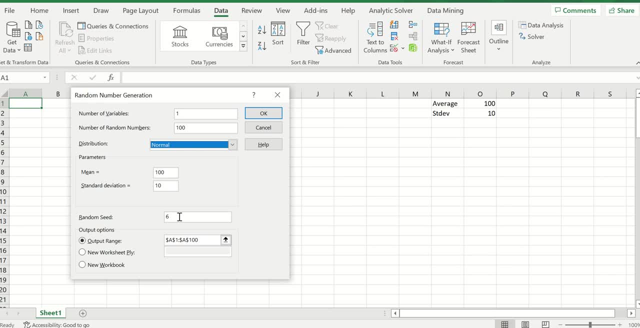 There's an algorithm in here for generating random numbers, but it wants a seed And so you put in whatever seed you want. I put six here. I'm doing I'm producing 100 random numbers, My output range. I want it here on this page. 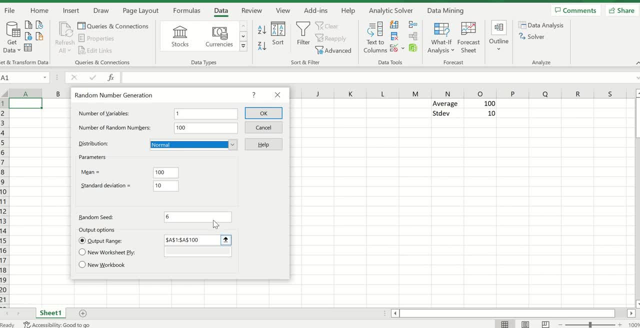 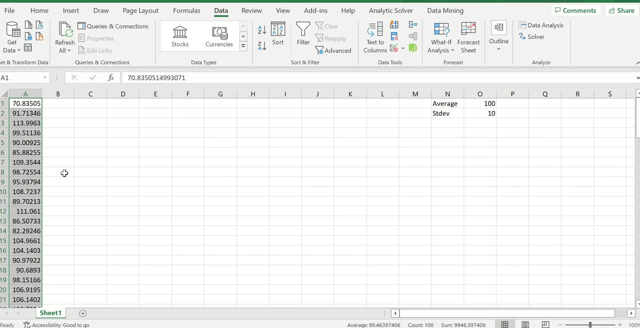 So I've gone A1 through A100, and I've input this information. I'm going to click OK. And lo and behold, Excel produces numbers for me. Okay, It produces how many numbers? Well, it produces 100 numbers. 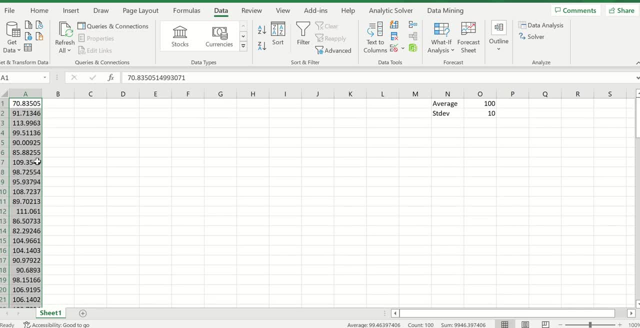 Just like I told it to produce in there. Okay, Now, what do these numbers mean to me? First of all, if this was monthly, demands these numbers really, since they're generated here, let me go back up here to the top. 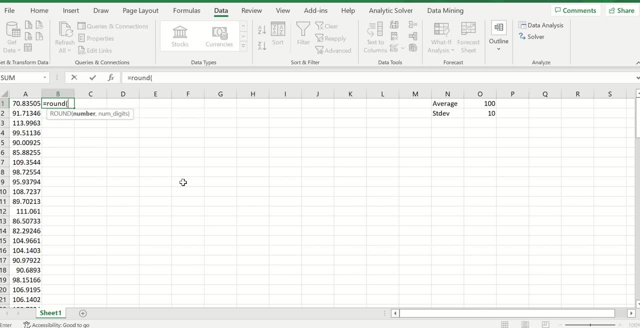 Let's round these numbers so that they make sense that they're integers. So I'm going to round this number. I don't need any decimal points, so I'm just going to tell it to give me zero decimal points, Hit enter, copy that down through there and then finally just to make this locked down. 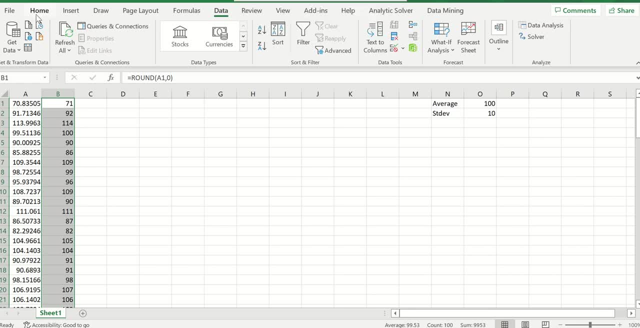 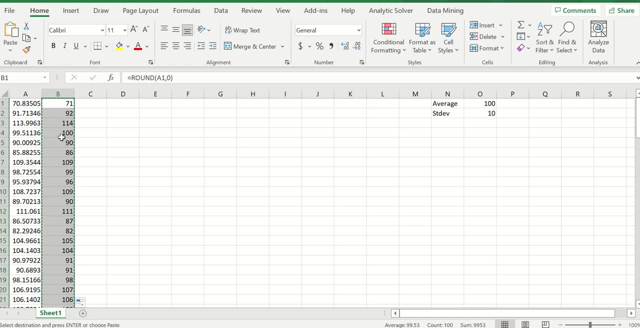 I'm going to copy it with a Control-C and then I'm just going to paste it back in as values And at that point I have 100 random numbers. What do these random numbers even mean? It says we don't know what the future is going to look like. 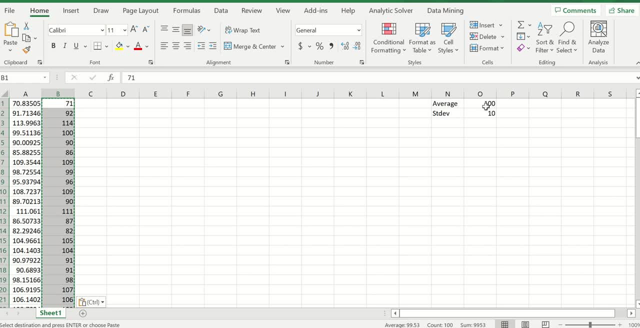 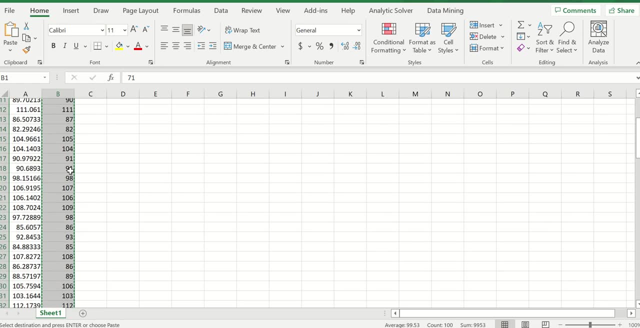 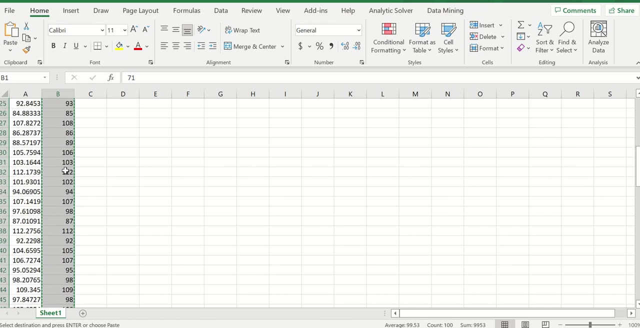 However, in the past we have an average of 100 per month, a standard deviation of 10.. One simulation using this information produces these possible outcomes for next month. It doesn't say it's the number, It doesn't say that it's correct. 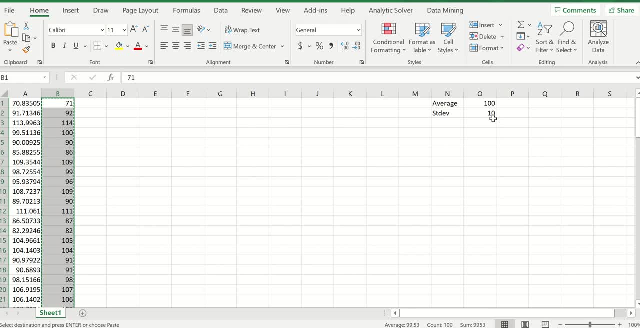 It just says that on a random number generator, if you have a number with this information, that any one of these 100 numbers could come up next month. How does that matter to us? Let's take the average. I'm going to put average here. 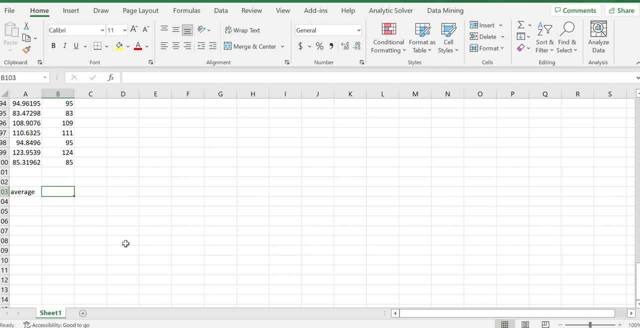 Because if I'm telling the boss, I've already gone through this stuff. I've told you where we've been, I've told you where I think we're going with my predictive, And now I need to use my prescriptive to be able to tell you. 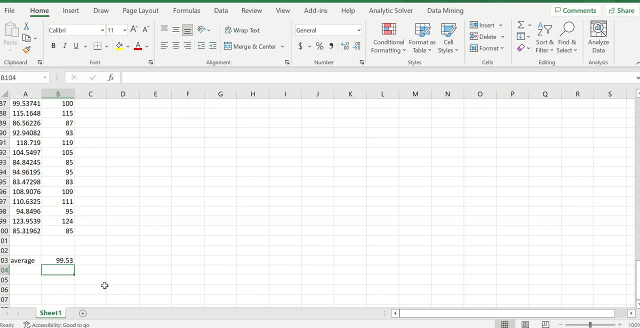 what should we do? Our random number generator has generated numbers that turn out to be an average of 99.5.. Well, guess what? That shouldn't be too much of a surprise, since we wanted it to give us an average of about 100. 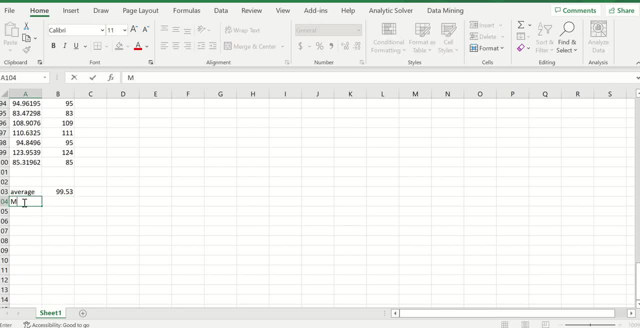 So we're happy there. Look at this. Look what happens whenever I do minimum. right, If I want the minimum, it may be a value to the boss, So I need to know That. the odds are that next month the number of demands will not likely be below 71.. 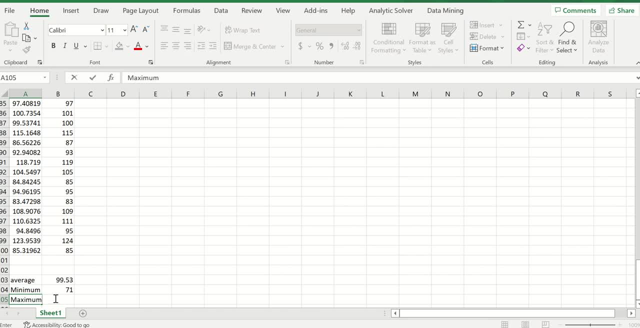 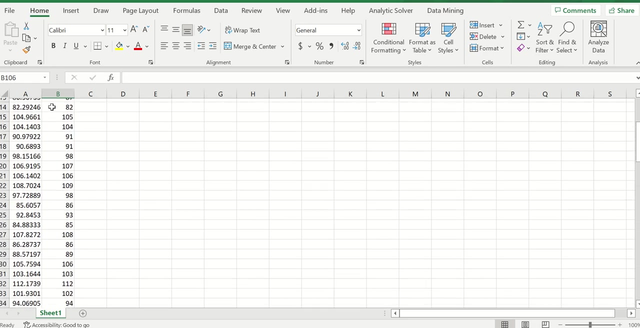 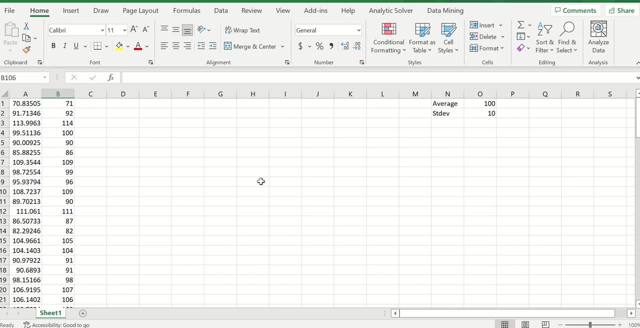 All right, maybe that's the value. What about maximum? Okay, so it's likely that the maximum won't be above 124.. So, based on simulation of a hundred events, based on a hundred events, using our normal distribution. so, once again, what i'm what it's trying to tell us is: 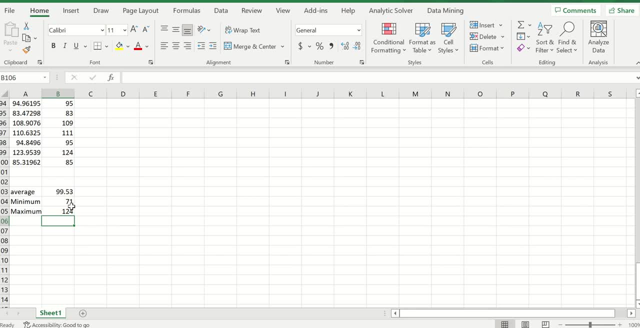 on the prescriptive side. i've done a monte carlo simulation. i have predicted with a hundred iterations that the average next month will be 99.5 or 100. the minimum is going to be around 71, maximum approximately 124.. again, it kind of just gives the boss some boundaries. it says we may not. 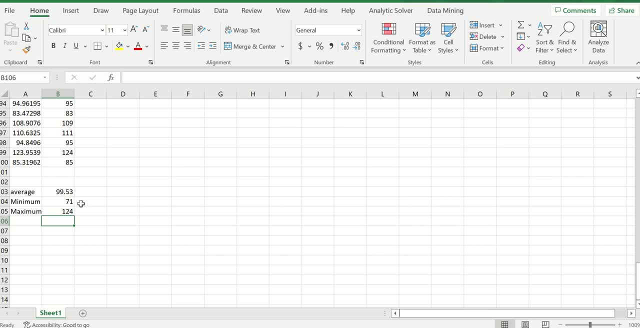 be right with a hundred. odds are we won't be below this. odds are we won't be above that. let's do this one more time. okay, if i go back in, if i've done 100 in this random sample, i could do this again. right, i could come in and i could say: 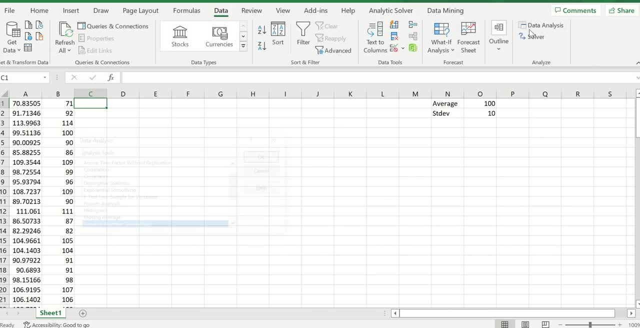 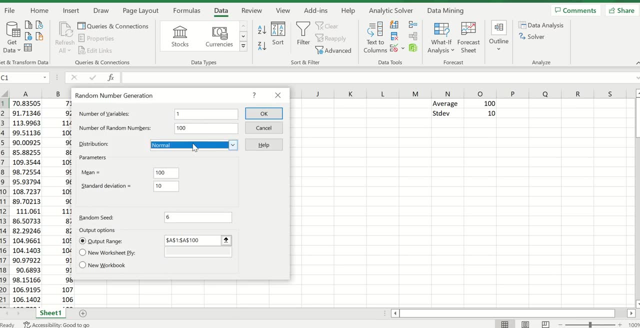 let's do back to my data data analysis. we're going to do random number generator- again same thing. i want another 100 use, normal distribution, same information as before. what's going to happen if i leave this seed as six, and here i'm going to change this now to: 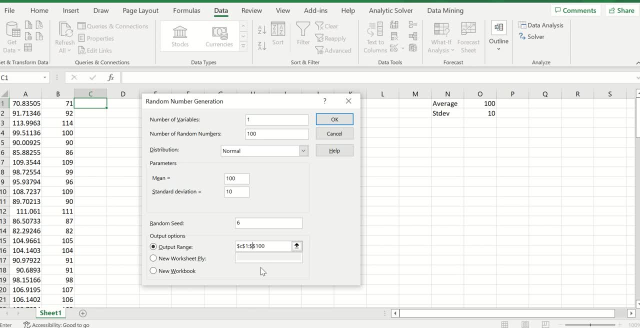 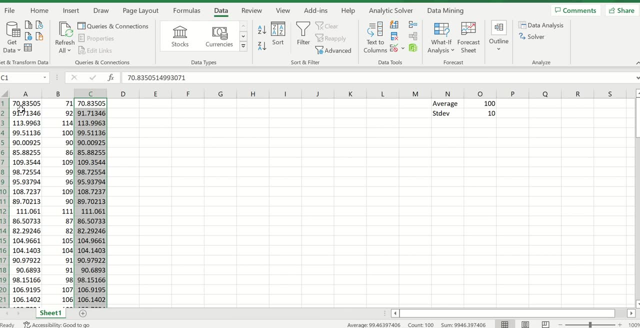 i'm going to generate this in column c. if i don't change the seed, i get exactly the same numbers i got right, so that doesn't make any sense to us. that's that is not helpful. instead, and once they're generated, they're set when we go back in there. 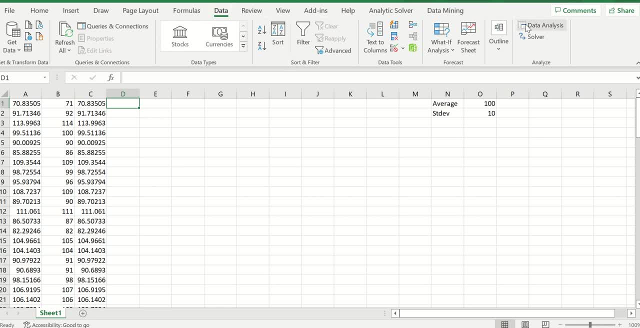 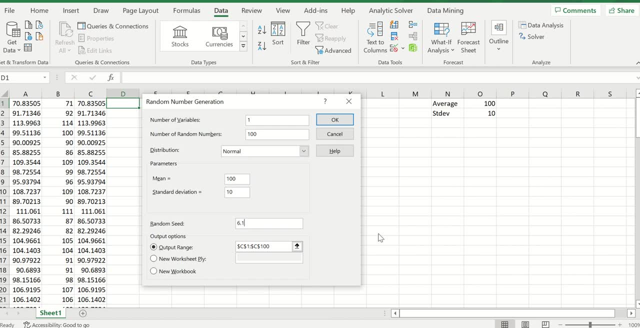 this time let's do data, data analysis, random number generator. let's change the seed just a little. even you can change it to a big number if you want. let's go ahead and tell it to overwrite c again. yeah, no, let's move it to d, just so we can see the 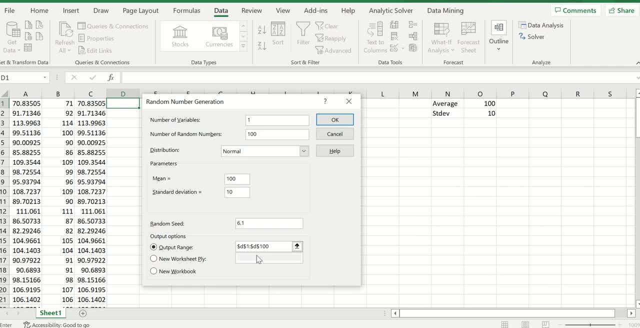 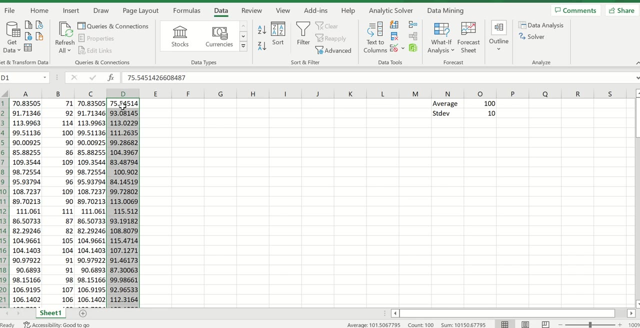 difference even easier. oh, it doesn't like the 0.1, so let's change it to 61 as the seed you could actually have, if are anyways regular or not. and now we've got the globaljin process and that's okay, they're having their own moon. well, it's not gonna extend or shift that way. so this is what we're testing right now. if you and i do the somersault here and we give you an example of what we've done and what's going on right now, this is something that we've done a long time ago- a few years ago- and it's almost quiet. much less any of our students remember overriding scaling in order to get that figure right into this box here. it is right below this bar. you just want to justCan i move this number 4.7. this is 1.3 and this is 1.9. all right, numbers are different. there's a different flow to it. this is 4.7 points higher than this. this is 1. 80. so you can see that these numbers really are random. go in, i'm going to do a round on this. equals round. 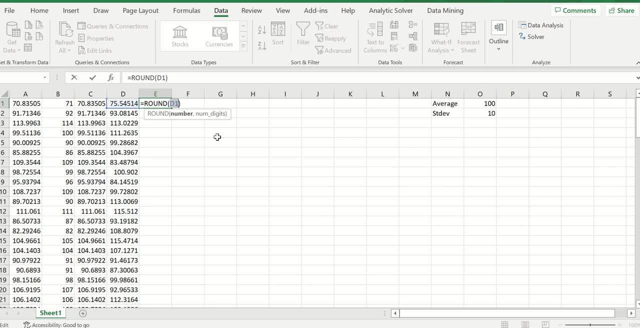 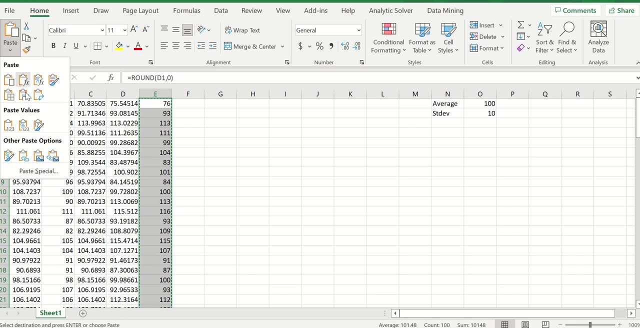 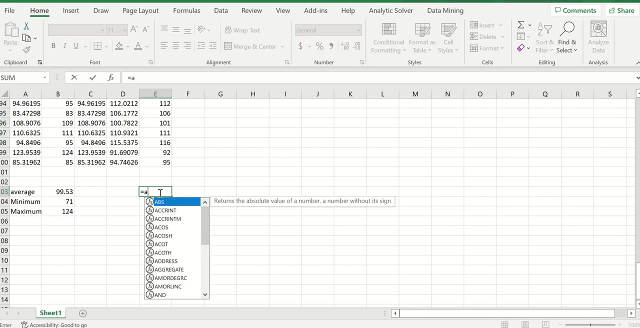 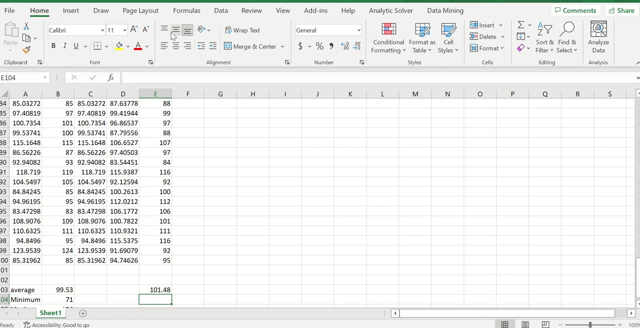 this value, 45%, I forgot to put in here, round it with zero decimals. copy it, paste it back in as just values. Let's go down here now and say, okay, what's the average for this? what's the minimum? 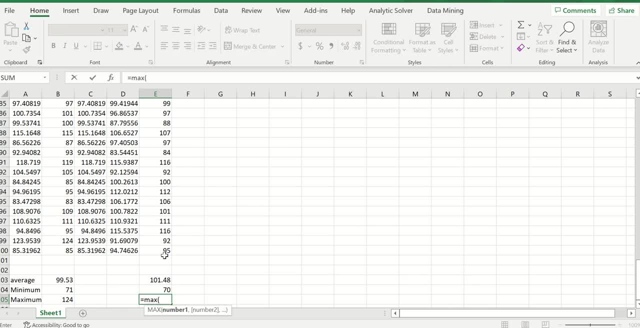 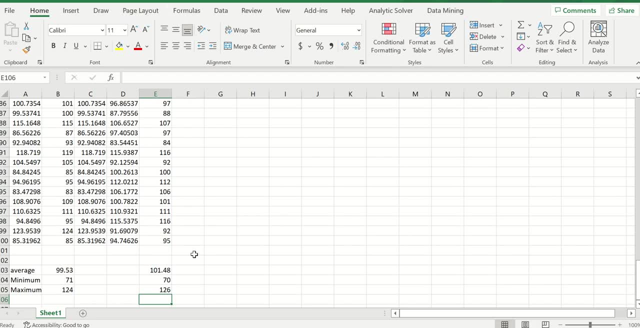 what's the maximum. All right, now we're beginning to see once again: if I did this several more times, look how much more certain we could look at the boss and say: the first time I did this, we never got below 70,. second time I did it, we never went below 70,. first time I did it. 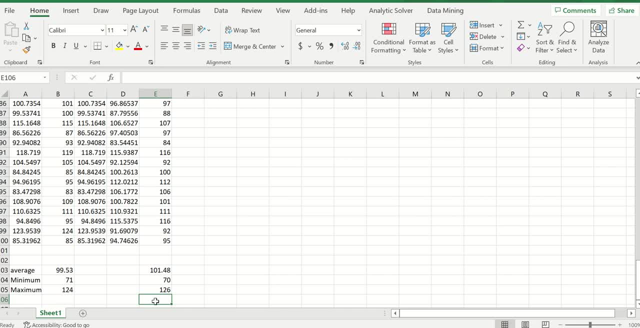 I never went above 124,. second time I never went above 126.. You see, if you did these, this simulation over, you know 10,, 12,, 13,, 14,, 15,, 16,, 17,. 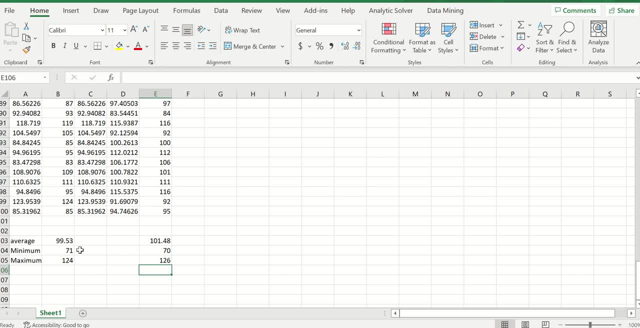 18,, 19,, 20 times that you would be able to start having with much more confidence to be able to tell the boss you know, even whenever I let the world be random as much as possible using our average and standard deviation, we still never fly off the page, right.